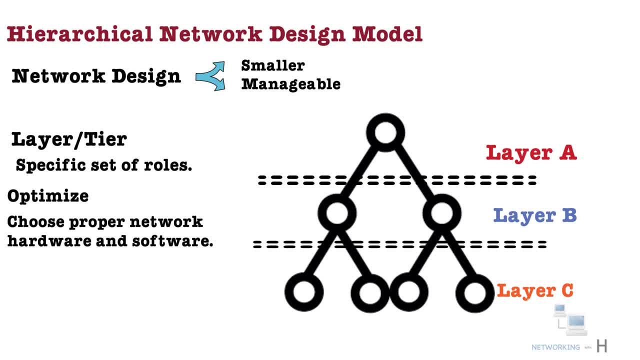 The two proven hierarchical design architecture for campus networks are three-tier model and two-tier model. A typical enterprise hierarchical campus network design includes the following three layers: core layer, distribution layer and the access layer. Three-tier model includes all the three layers. This design model can be used in large campus networks. 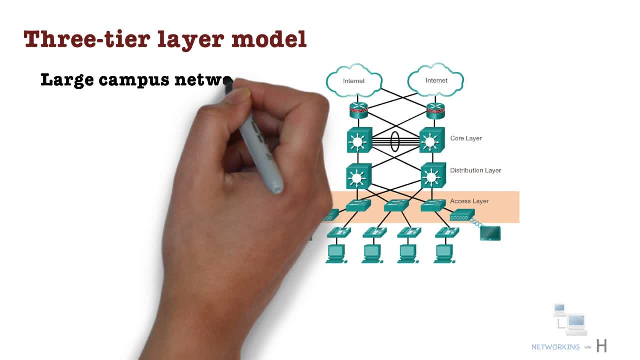 This design model can be used in large campus networks. This design model can be used in large campus networks Where multiple distribution layer and building needs to be interconnected. Where multiple distribution layer and building needs to be interconnected, Let's begin with the access layer. 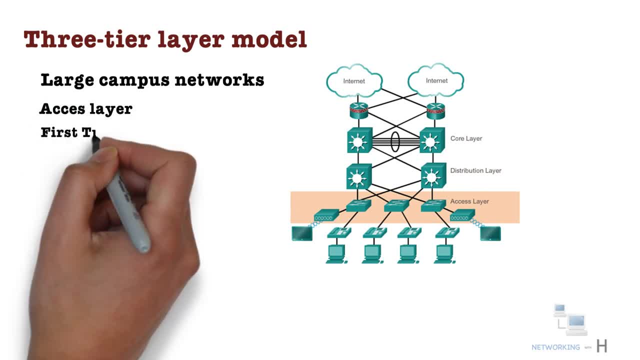 Let's begin with the access layer. The access layer is the first tier, or edge of the campus. The access layer is the first tier, or edge, of the campus. It grants end devices access to the network. It grants end devices access to the network. 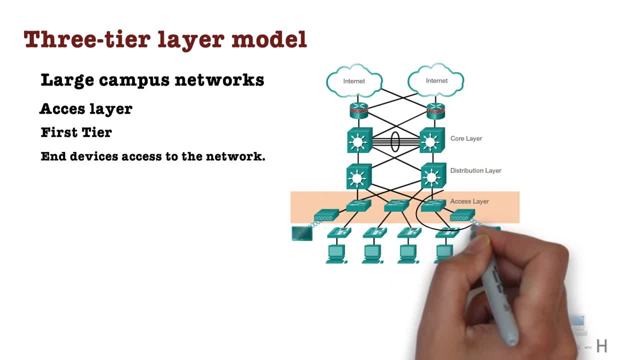 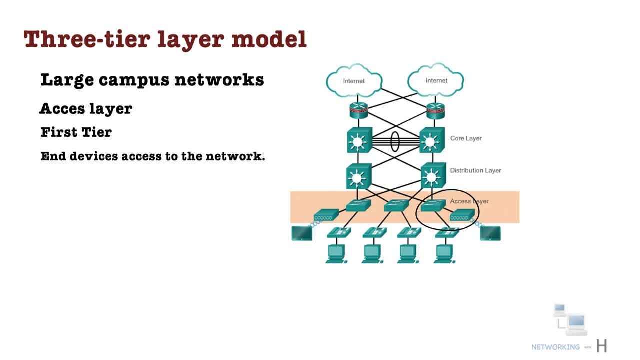 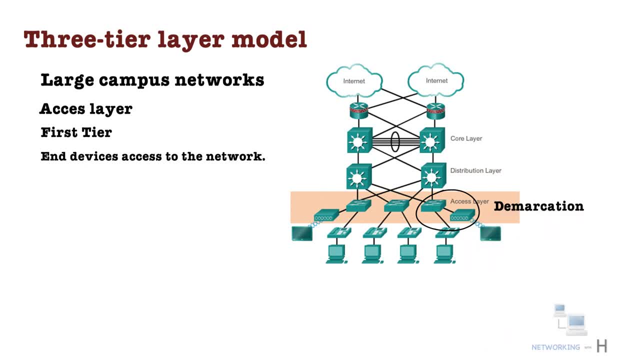 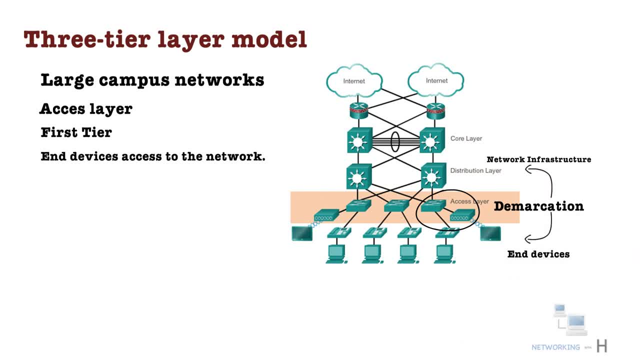 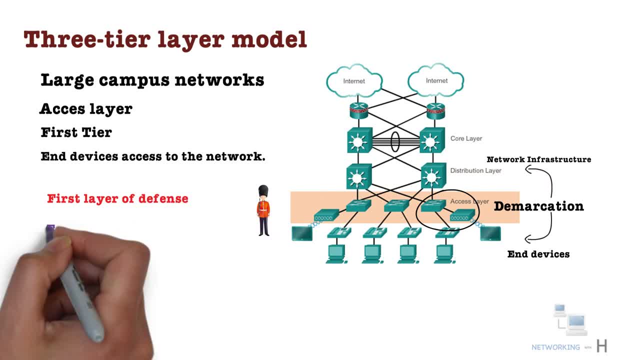 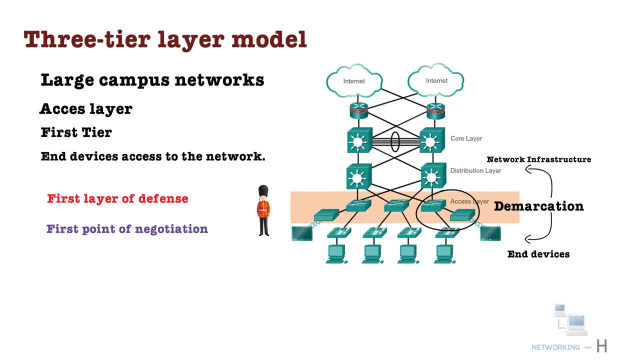 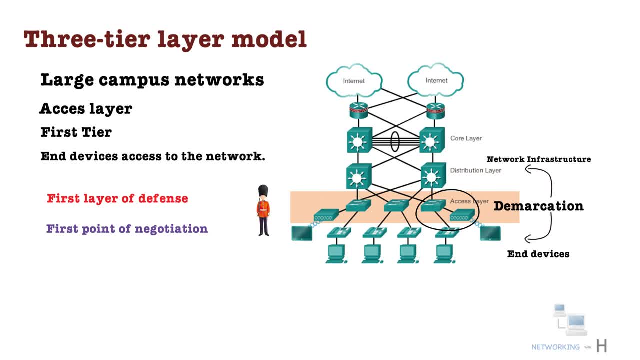 When looking at the overall campus design, the access switch provides the majority of these access layer services and is a key element in enabling multiple campus services. When looking at the overall campus design, the access switch provides the majority of these access layer services and is a key element in enabling multiple campus services. 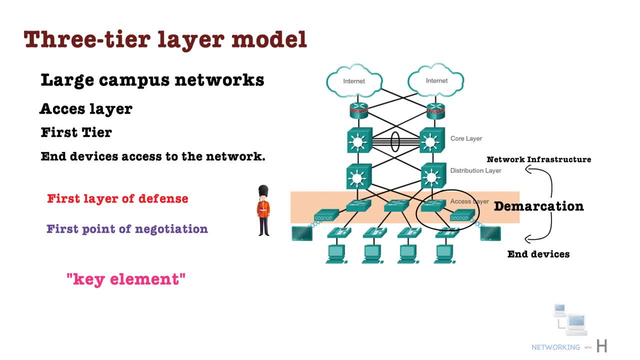 When looking at the overall campus design, the access switch provides the majority of these access layer services and is a key element in enabling multiple campus services. When looking at the overall campus design, the access switch provides the majority of these access layer services and is a key element in enabling multiple campus services. 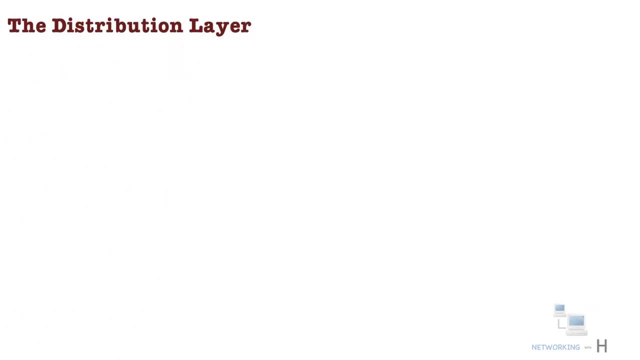 When looking at the overall campus design, the access switch provides the majority of these access layer services and is a key element in enabling multiple campus services. When looking at the overall campus design, the access switch provides the majority of these access layer services and is a key element in enabling multiple campus services. 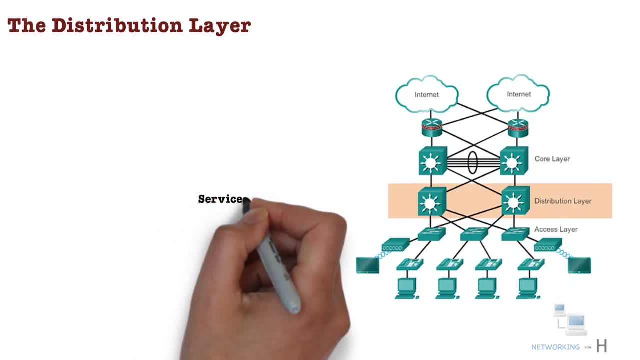 When looking at the overall campus design, the access switch provides the majority of these access layer services and is a key element in enabling multiple campus services. When looking at the overall campus design, the access switch provides the majority of these access layer services and is a key element in enabling multiple campus services. 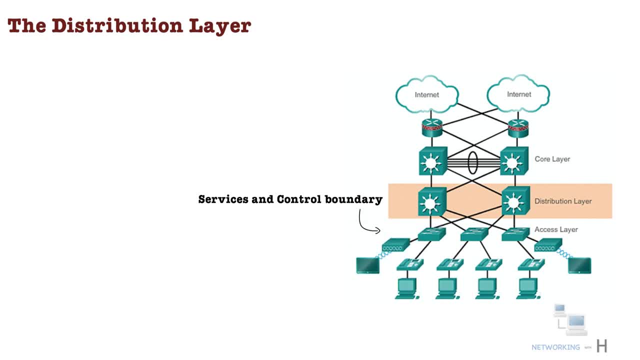 When looking at the overall campus design, the access switch provides the majority of these access layer services and is a key element in enabling multiple campus services. When looking at the overall campus design, the access switch provides the majority of these access layer services and is a key element in enabling multiple campus services. 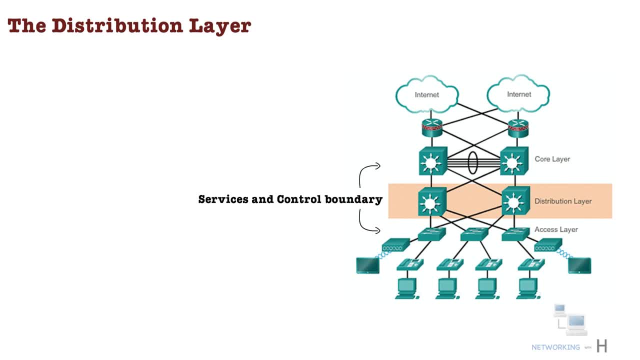 When looking at the overall campus design, the access switch provides the majority of these access layer services and is a key element in enabling multiple campus services. When looking at the overall campus design, the access switch provides the majority of these access layer services and is a key element in enabling multiple campus services. 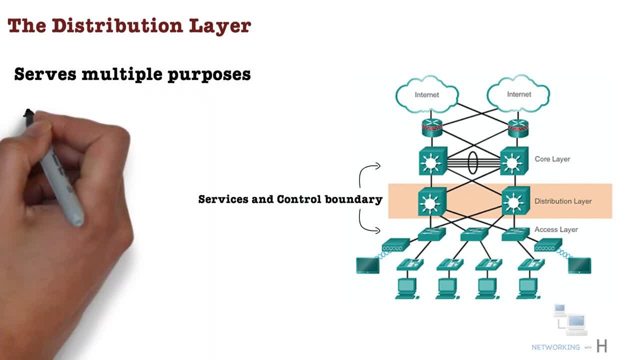 When looking at the overall campus design, the access switch provides the majority of these access layer services and is a key element in enabling multiple campus services. When looking at the overall campus design, the access switch provides the majority of these access layer services and is a key element in enabling multiple campus services. 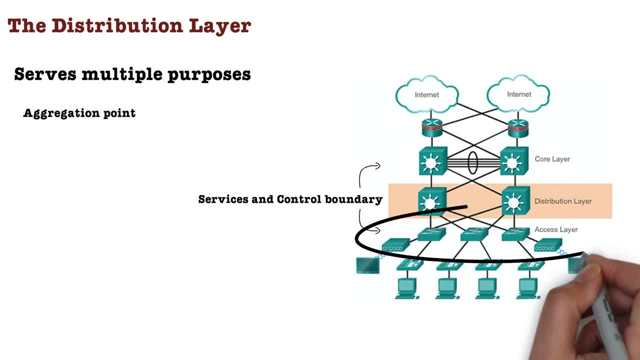 When looking at the overall campus design, the access switch provides the majority of these access layer services and is a key element in enabling multiple campus services. When looking at the overall campus design, the access switch provides the majority of these access layer services and is a key element in enabling multiple campus services. 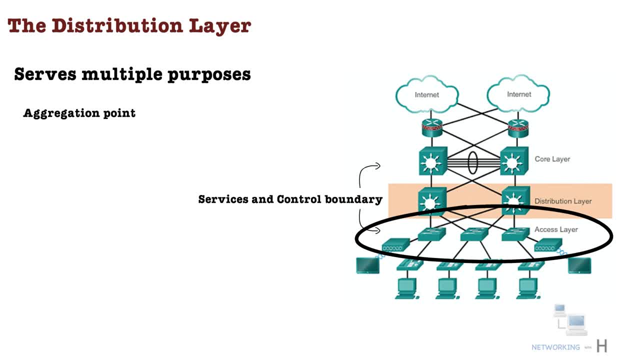 When looking at the overall campus design, the access switch provides the majority of these access layer services and is a key element in enabling multiple campus services. When looking at the overall campus design, the access switch provides the majority of these access layer services and is a key element in enabling multiple campus services. 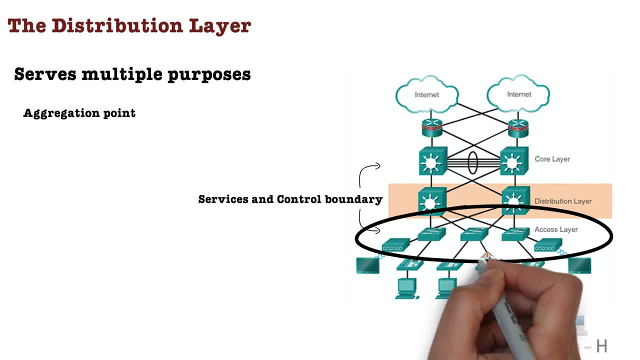 When looking at the overall campus design, the access switch provides the majority of these access layer services and is a key element in enabling multiple campus services. When looking at the overall campus design, the access switch provides the majority of these access layer services and is a key element in enabling multiple campus services. 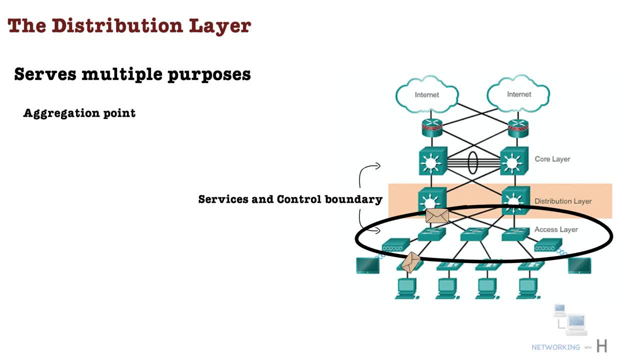 When looking at the overall campus design, the access switch provides the majority of these access layer services and is a key element in enabling multiple campus services. When looking at the overall campus design, the access switch provides the majority of these access layer services and is a key element in enabling multiple campus services. 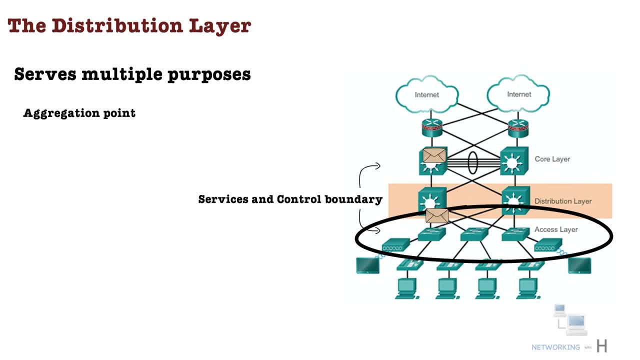 When looking at the overall campus design, the access switch provides the majority of these access layer services and is a key element in enabling multiple campus services. When looking at the overall campus design, the access switch provides the majority of these access layer services and is a key element in enabling multiple campus services. 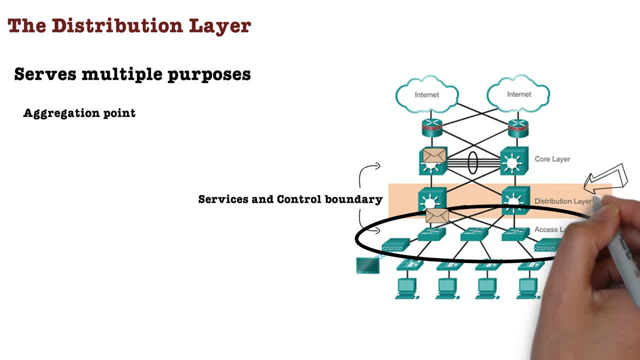 When looking at the overall campus design, the access switch provides the majority of these access layer services and is a key element in enabling multiple campus services. When looking at the overall campus design, the access switch provides the majority of these access layer services and is a key element in enabling multiple campus services. 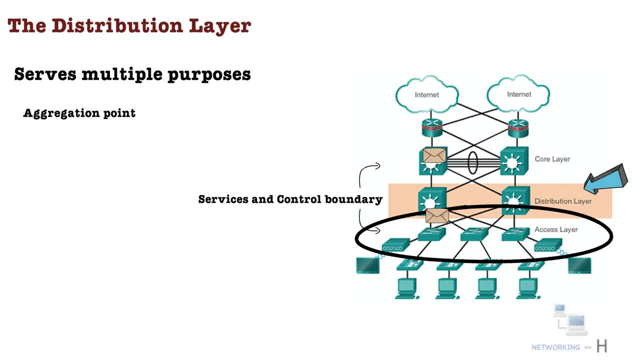 When looking at the overall campus design, the access switch provides the majority of these access layer services and is a key element in enabling multiple campus services. When looking at the overall campus design, the access switch provides the majority of these access layer services and is a key element in enabling multiple campus services. 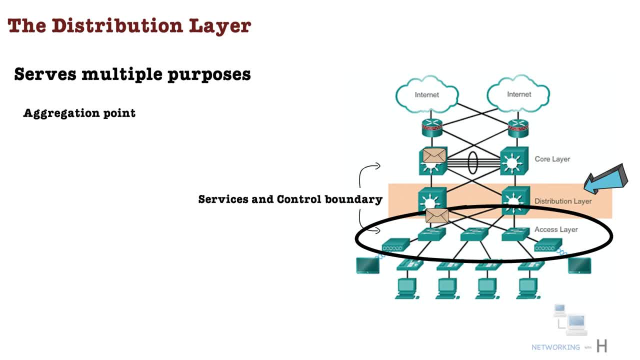 When looking at the overall campus design, the access switch provides the majority of these access layer services and is a key element in enabling multiple campus services. When looking at the overall campus design, the access switch provides the majority of these access layer services and is a key element in enabling multiple campus services. 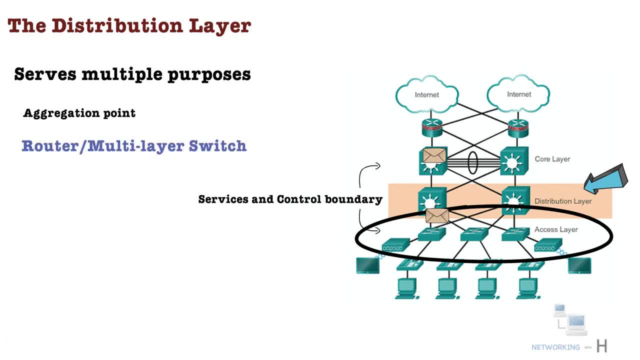 When looking at the overall campus design, the access switch provides the majority of these access layer services and is a key element in enabling multiple campus services. When looking at the overall campus design, the access switch provides the majority of these access layer services and is a key element in enabling multiple campus services. 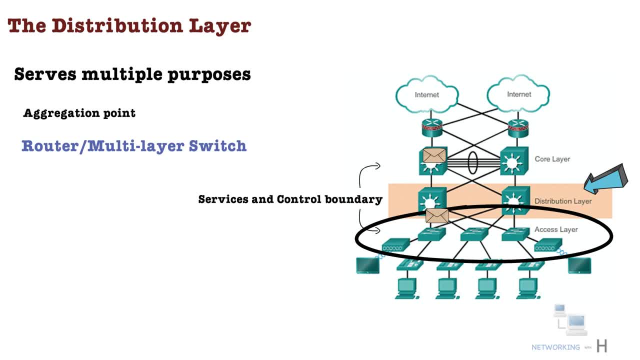 When looking at the overall campus design, the access switch provides the majority of these access layer services and is a key element in enabling multiple campus services. When looking at the overall campus design, the access switch provides the majority of these access layer services and is a key element in enabling multiple campus services. 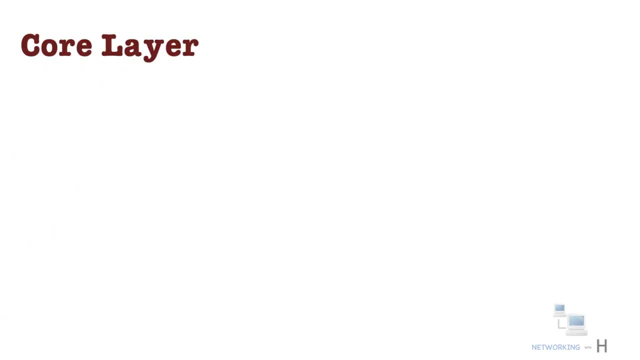 When looking at the overall campus design, the access switch provides the majority of these access layer services and is a key element in enabling multiple campus services. When looking at the overall campus design, the access switch provides the majority of these access layer services and is a key element in enabling multiple campus services. 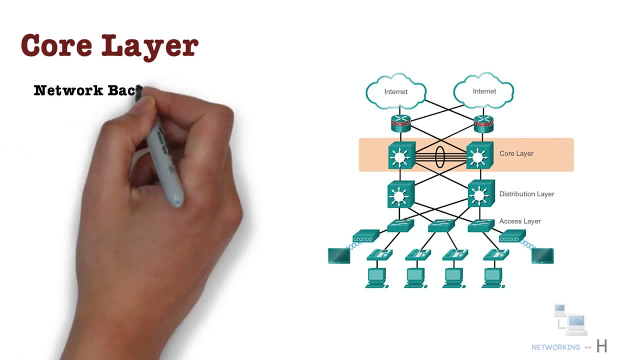 When looking at the overall campus design, the access switch provides the majority of these access layer services and is a key element in enabling multiple campus services. When looking at the overall campus design, the access switch provides the majority of these access layer services and is a key element in enabling multiple campus services. 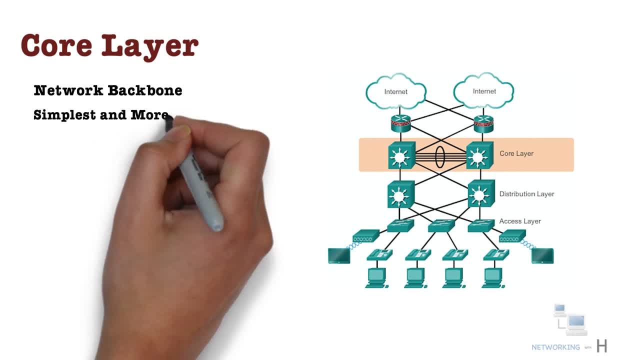 When looking at the overall campus design, the access switch provides the majority of these access layer services and is a key element in enabling multiple campus services. When looking at the overall campus design, the access switch provides the majority of these access layer services and is a key element in enabling multiple campus services. 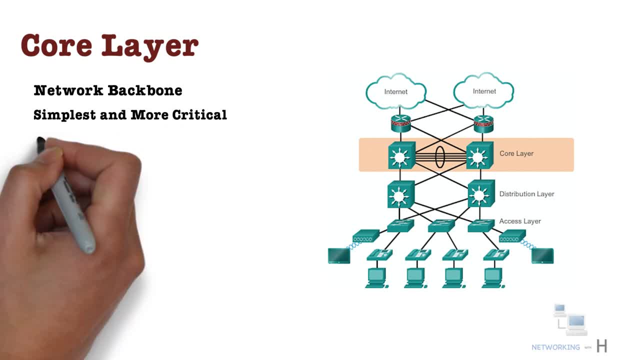 When looking at the overall campus design, the access switch provides the majority of these access layer services and is a key element in enabling multiple campus services. When looking at the overall campus design, the access switch provides the majority of these access layer services and is a key element in enabling multiple campus services. 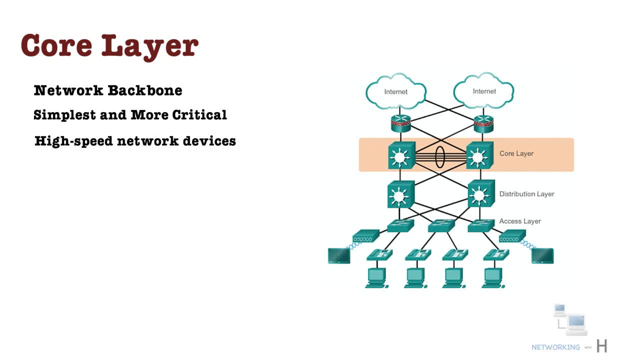 When looking at the overall campus design, the access switch provides the majority of these access layer services and is a key element in enabling multiple campus services. When looking at the overall campus design, the access switch provides the majority of these access layer services and is a key element in enabling multiple campus services. 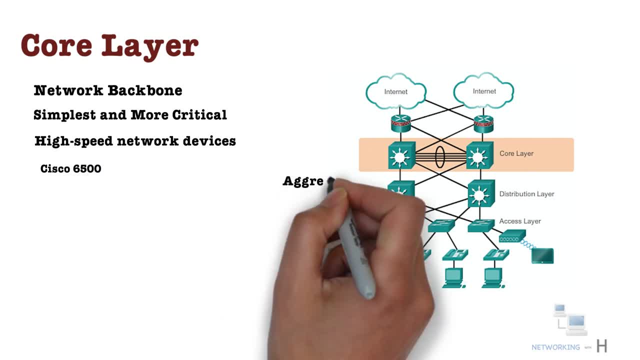 When looking at the overall campus design, the access switch provides the majority of these access layer services and is a key element in enabling multiple campus services. When looking at the overall campus design, the access switch provides the majority of these access layer services and is a key element in enabling multiple campus services. 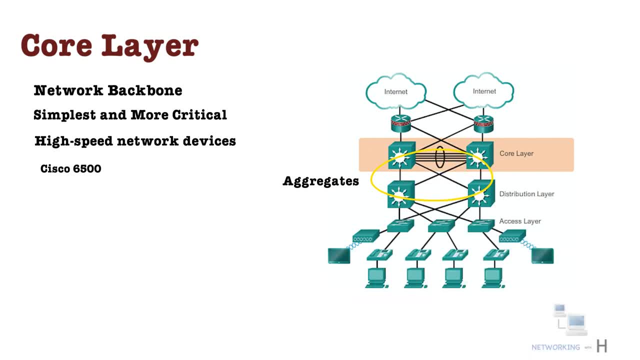 When looking at the overall campus design, the access switch provides the majority of these access layer services and is a key element in enabling multiple campus services. When looking at the overall campus design, the access switch provides the majority of these access layer services and is a key element in enabling multiple campus services. 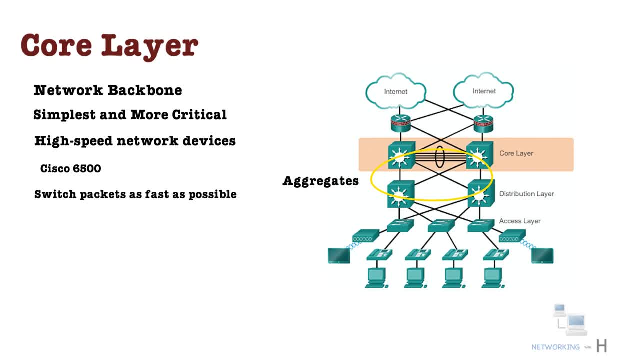 When looking at the overall campus design, the access switch provides the majority of these access layer services and is a key element in enabling multiple campus services. When looking at the overall campus design, the access switch provides the majority of these access layer services and is a key element in enabling multiple campus services. 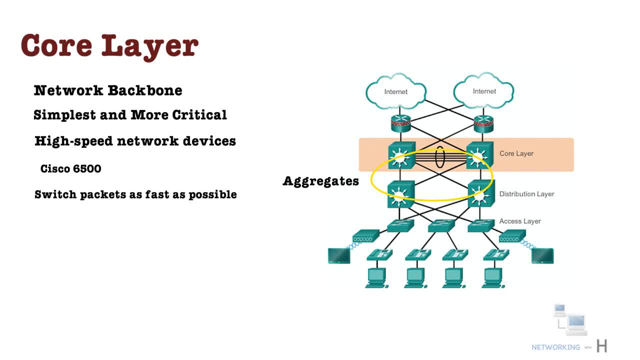 When looking at the overall campus design, the access switch provides the majority of these access layer services and is a key element in enabling multiple campus services. When looking at the overall campus design, the access switch provides the majority of these access layer services and is a key element in enabling multiple campus services. 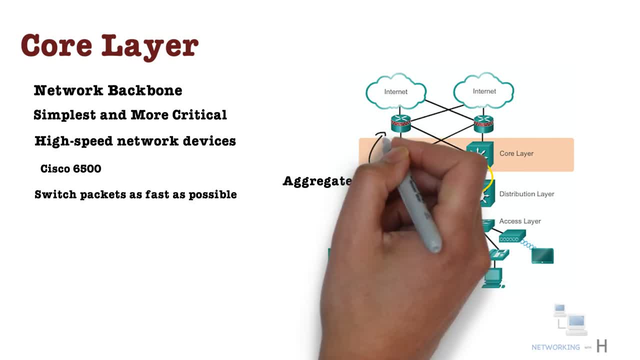 When looking at the overall campus design, the access switch provides the majority of these access layer services and is a key element in enabling multiple campus services. When looking at the overall campus design, the access switch provides the majority of these access layer services and is a key element in enabling multiple campus services. 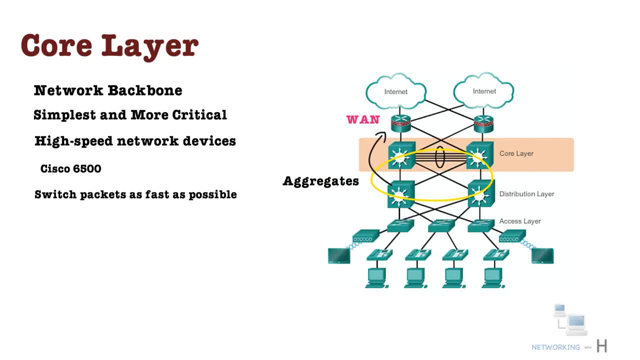 When looking at the overall campus design, the access switch provides the majority of these access layer services and is a key element in enabling multiple campus services. When looking at the overall campus design, the access switch provides the majority of these access layer services and is a key element in enabling multiple campus services. 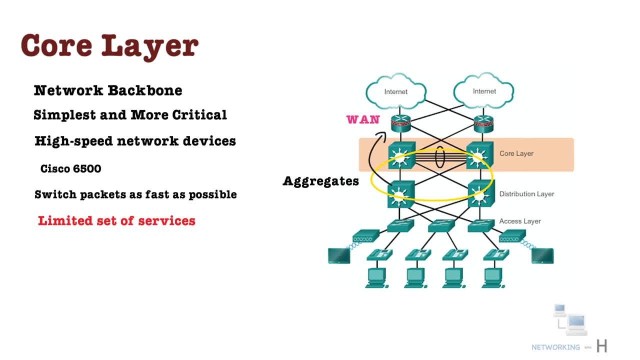 When looking at the overall campus design, the access switch provides the majority of these access layer services and is a key element in enabling multiple campus services. When looking at the overall campus design, the access switch provides the majority of these access layer services and is a key element in enabling multiple campus services. 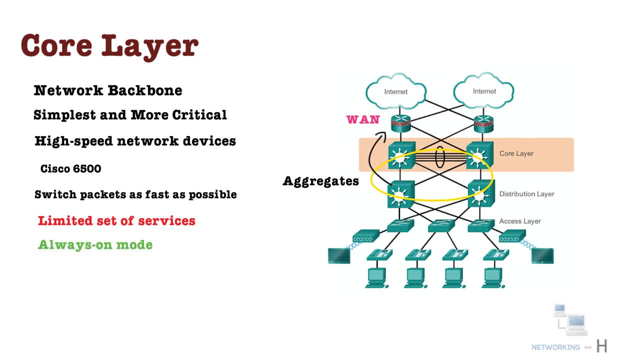 When looking at the overall campus design, the access switch provides the majority of these access layer services and is a key element in enabling multiple campus services. When looking at the overall campus design, the access switch provides the majority of these access layer services and is a key element in enabling multiple campus services. 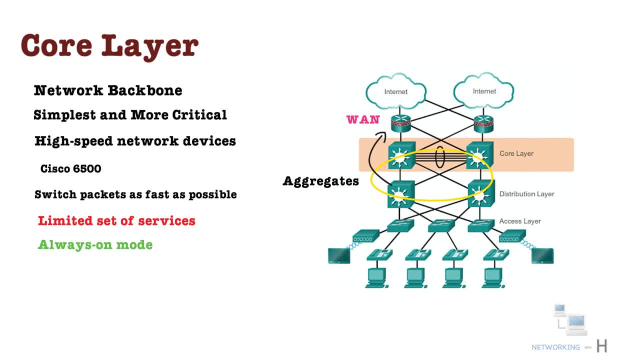 When looking at the overall campus design, the access switch provides the majority of these access layer services and is a key element in enabling multiple campus services. When looking at the overall campus design, the access switch provides the majority of these access layer services and is a key element in enabling multiple campus services. 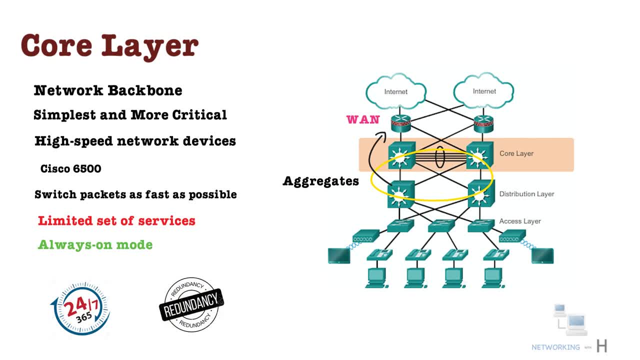 When looking at the overall campus design, the access switch provides the majority of these access layer services and is a key element in enabling multiple campus services. When looking at the overall campus design, the access switch provides the majority of these access layer services and is a key element in enabling multiple campus services. 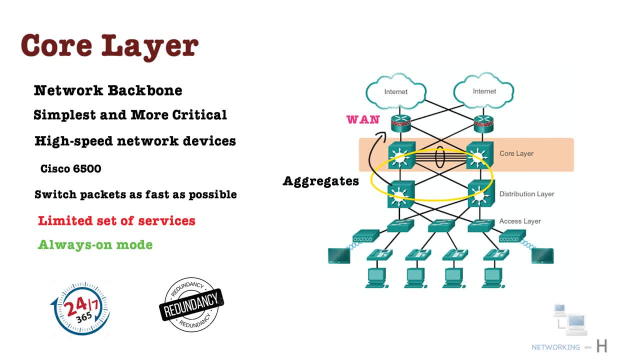 When looking at the overall campus design, the access switch provides the majority of these access layer services and is a key element in enabling multiple campus services. When looking at the overall campus design, the access switch provides the majority of these access layer services and is a key element in enabling multiple campus services. 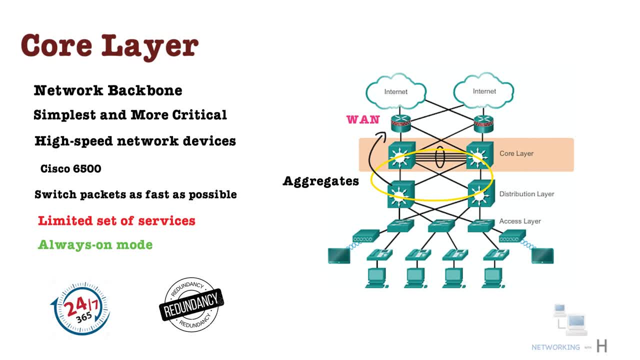 When looking at the overall campus design, the access switch provides the majority of these access layer services and is a key element in enabling multiple campus services. When looking at the overall campus design, the access switch provides the majority of these access layer services and is a key element in enabling multiple campus services. 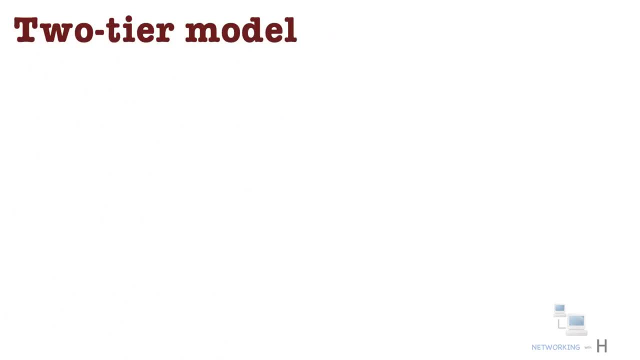 When looking at the overall campus design, the access switch provides the majority of these access layer services and is a key element in enabling multiple campus services. When looking at the overall campus design, the access switch provides the majority of these access layer services and is a key element in enabling multiple campus services. 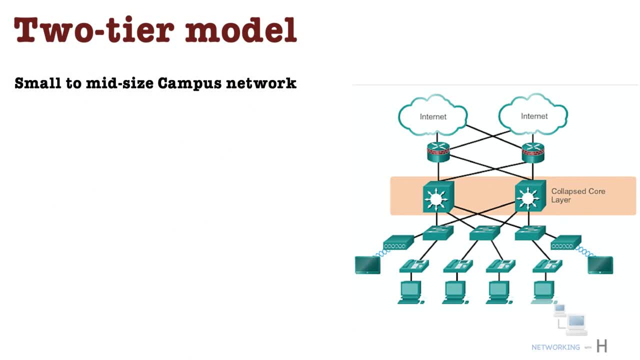 When looking at the overall campus design, the access switch provides the majority of these access layer services and is a key element in enabling multiple campus services. When looking at the overall campus design, the access switch provides the majority of these access layer services and is a key element in enabling multiple campus services. 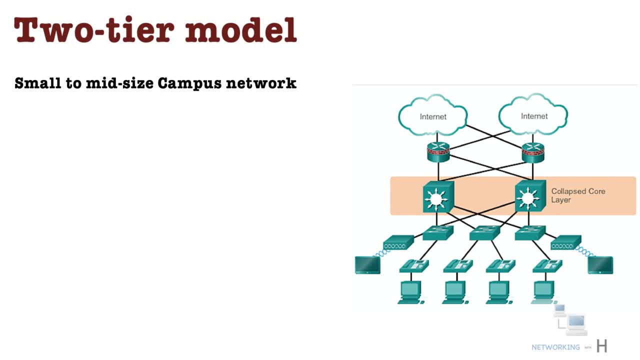 When looking at the overall campus design, the access switch provides the majority of these access layer services and is a key element in enabling multiple campus services. When looking at the overall campus design, the access switch provides the majority of these access layer services and is a key element in enabling multiple campus services.